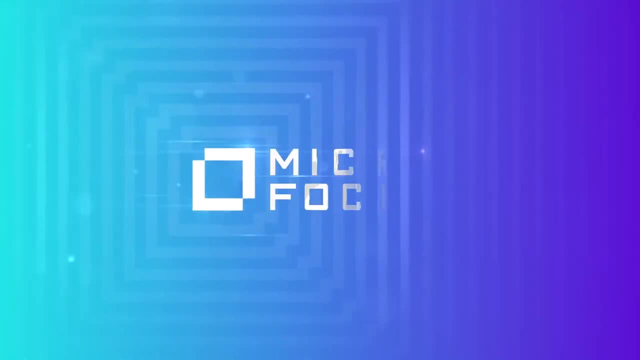 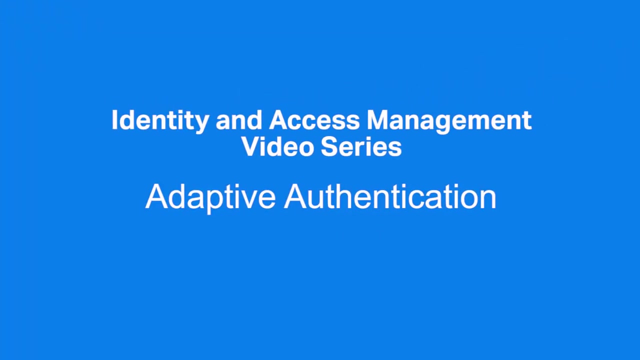 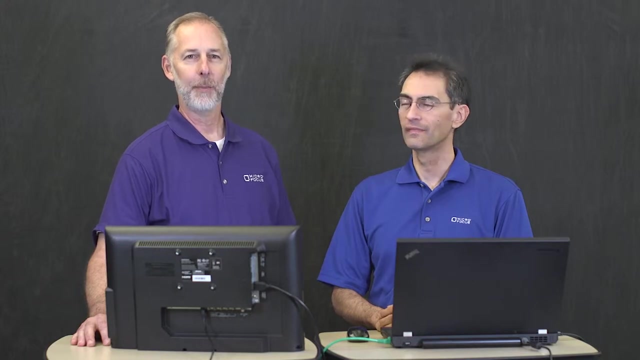 Hello everyone, welcome to the Micro Focus Identity and Access Management video series. I'm Kent Purdy, Product Marketing Manager for Access Management, And I'm Paul McKeith, Identity and Access Management Specialist from Micro Focus. In the other videos, we showed how Access Manager could deliver secure access through. 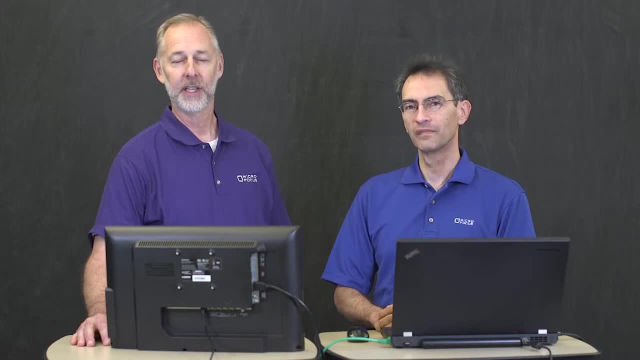 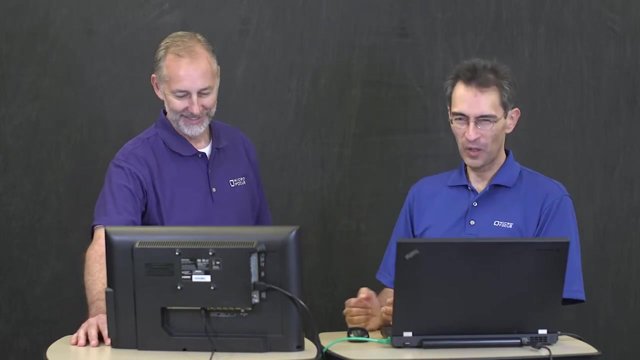 applications and services out in the cloud or in hybrid environments. In this video, we're going to show how to use the risk-based authentication feature in Access Manager to adapt the authentication type to the level of risk at hand. So you're telling me you'd like to see this, eh? Kent? 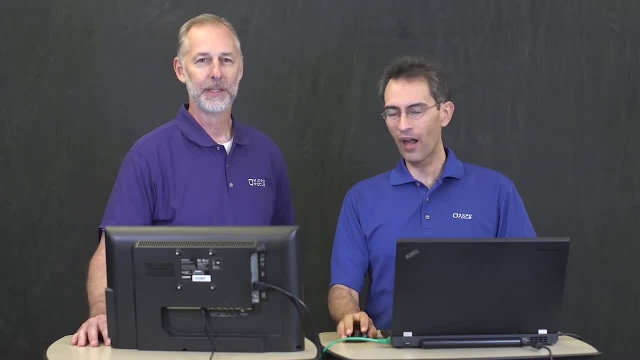 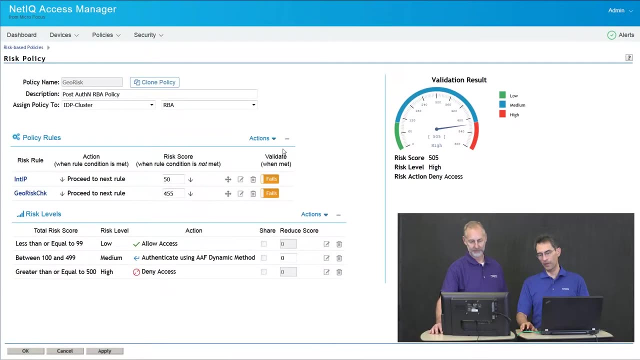 Okay, so let's go ahead and do that. I'll take us right into our administration console right from the start. So here you can see that we're in Access Manager. This is our default administration console, But I focused in on the risk-based policies and rules that will govern access from an. 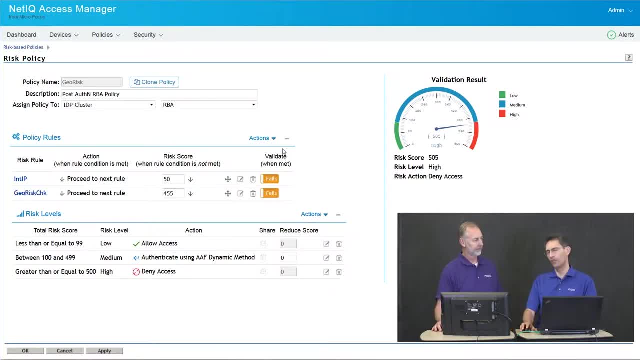 authentication perspective before people actually get access. So when they're authenticating, what kind of authentication are they going to need or require before we allow them into that particular application? So on this dashboard, what you're seeing is basically our risk policy. I can have a number of risk policies. 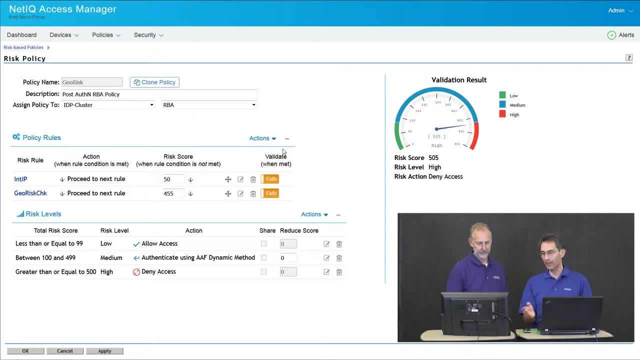 I can add those risk policies to different applications at different times for different purposes. I can mix and match what I need in terms of risk level to the application or what we're actually accessing. So, on this, what you're seeing is a couple of rules that I've already configured and 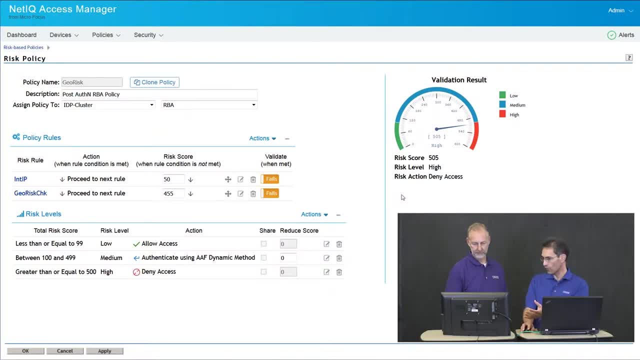 a dashboard here that tells you what's going to happen for the administrator that's going to build these. So, for example, if I go ahead and turn this rule onto a pass or a fail, you can see on the right how the access or the meter, the level, changes, and it actively does this. 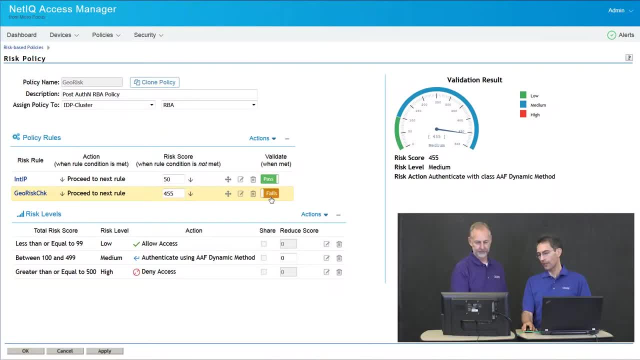 Yes, Kent. So what did that rule do When you switch that? Ah, that's a great question. So the very first rule in this one- this one's actually one to look at- am I from the internal or external network? 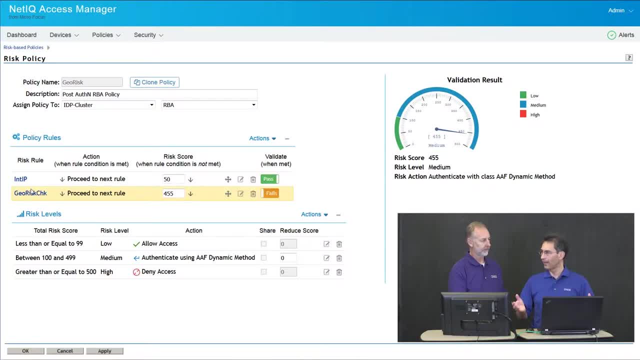 If I'm on the internal network I have more control over that right. It's the old. I'm inside the firewall. I've got lots of controls on devices access to the network, So I want to. that's a risk level that if you're outside the network I want to change. 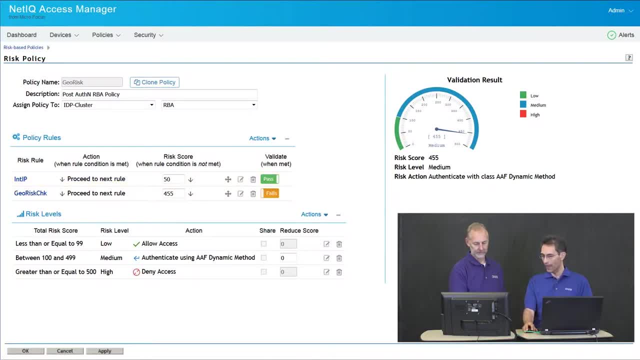 that risk level. So that's the first thing I'm checking here. So if I pass, you can see when this rule is met. then it's going to lower my risk score. You can see it's 455.. Right, If I'm outside, that's going to fail and that's 505, it increased my risk. 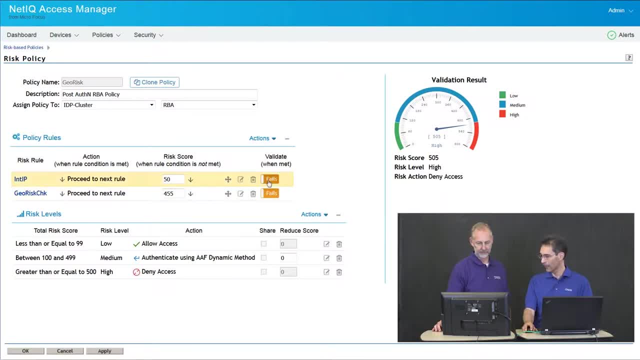 And you'll note that it also denied my access. But if I am on the inside of the network and I hit pass and then I check to my next rule. So my next rule is: not only am I going to see if I'm inside or outside the corporate, 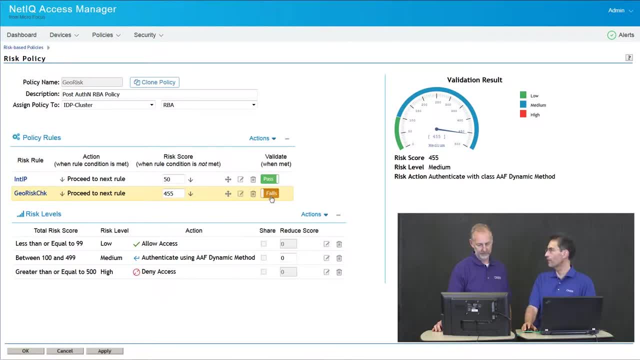 network. but where in the world am I coming from outside the corporate network? That might be for a North American based company, that may be specific to a state, a city, the whole country, Or for worldwide, it may be a lot more, you know. widespread availability. 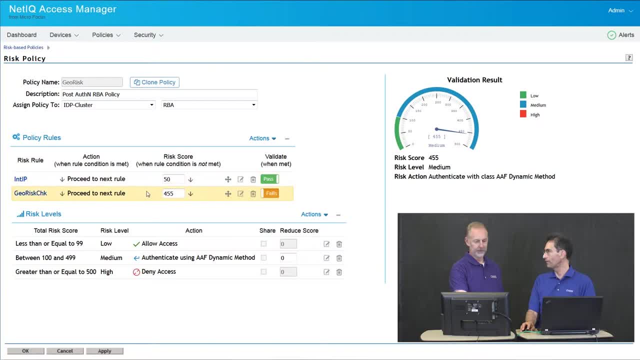 But still, that's a level of risk that I want to check, based on my business. So you have your inside the building or you're out and about traveling somewhere. What are the kind of rules can you build? We can build lots of rules, and I'm going to show you a bunch of those. 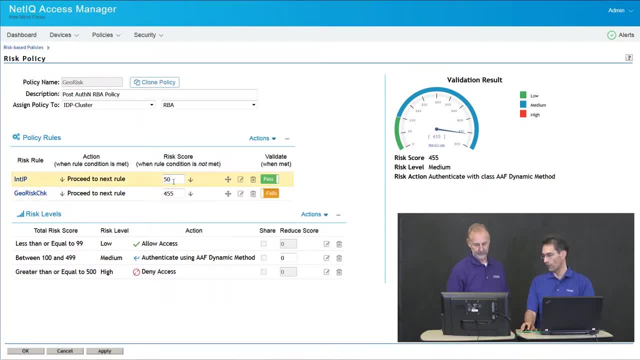 One thing to keep in mind here is that, as these rules are here, you see these risk scores And each one of these, as we pass and fail, you notice that they would do things right. We get access Okay, Based on the pass-fail. 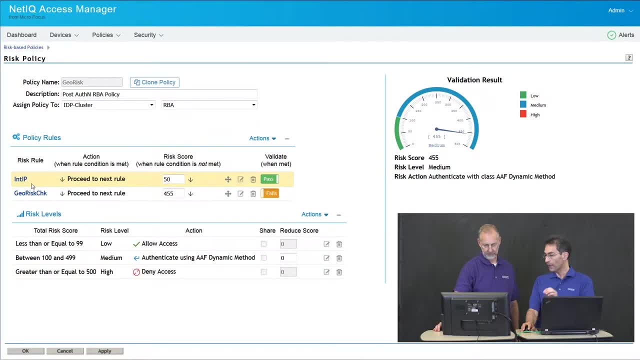 But they also categorize this risk into risk levels. So that's where I can build as many rules as I would like. calculate those assign a risk level to that particular scenario. So I can get really really complex or really really simple, like this, based on my risk posture. 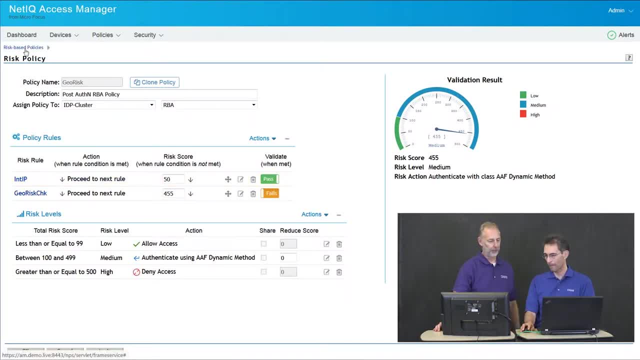 that I have for that particular application, So it could be one rule or half a dozen, whatever you need Exactly. That's perfect, right, Because we can put in as many rules as we need And again, I can have multiple policies and have a different policy for different things. 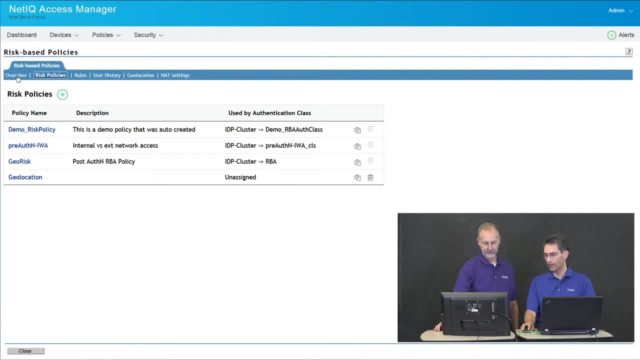 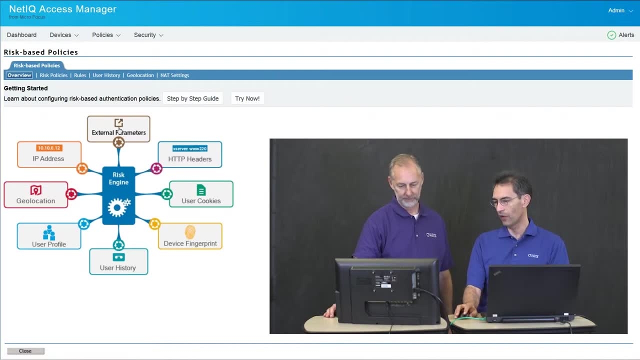 Okay, Different types of applications. So if I go up here and I take a look at all of the rules that I can, at my palette of rules that I can choose from, this is where we start. So I'll start over here. on the IP address. 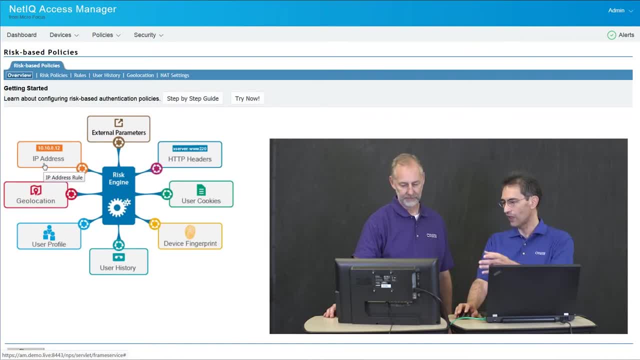 So that very first rule. you saw the internal IP address check. I can check and see where you're coming from. Are you an internal network address or are you an external network address? And I can build that policy And I can populate that from your network. 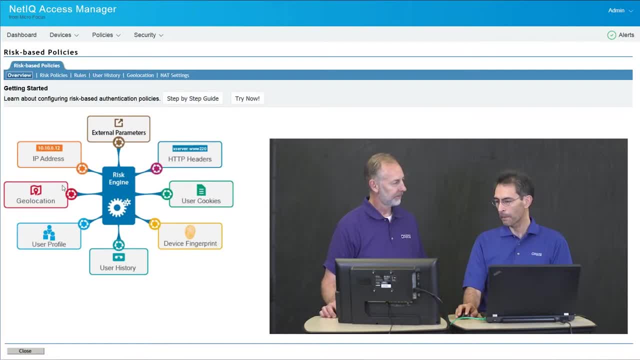 I can populate it from the administration council here a number of ways. Then that second rule in there was about geo-level, Geo-location, So geo-location, this is where I can go. okay, now I'm going to find out where this guy is. 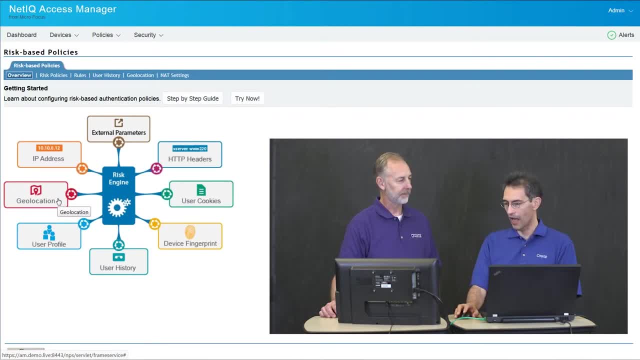 coming from and see if that's a risk that I'm willing to tolerate or not. The user profiles is okay. now that I've identified who the user is, is there something special about this particular user? For example, this bridges over a little bit into privilege access management, which really 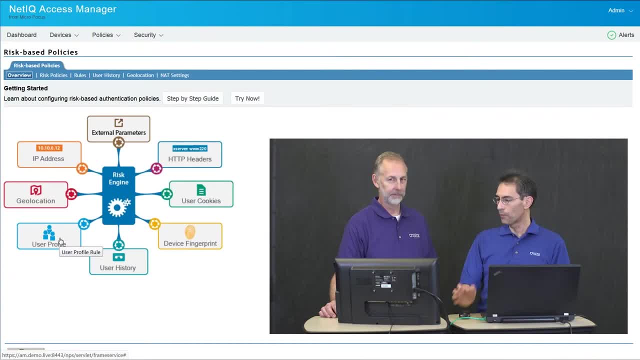 isn't what this is, but this augments that, in the sense that a privilege user, an administrator of a particular application, may get access only when he's on the internal network or if he's on the external network. I'm going to require an even more stringent rule set. 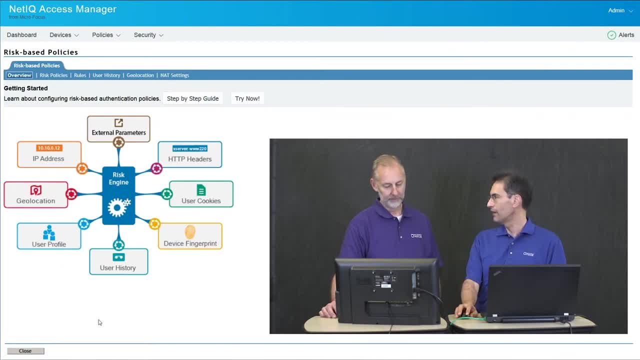 in order to allow him access, Or this just may be. you know I don't like Kent, so I'm going to create a rule that doesn't allow Kent into this application. There you go, As simple as you want, Exactly. 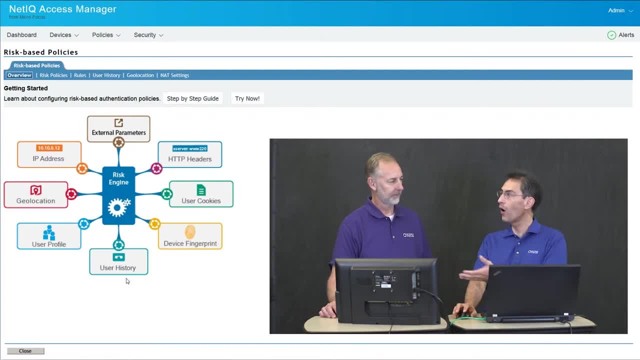 User history is a way for us to go look at the pattern of the past. So how often has Kent logged in? How often has he actually been granted access? Maybe if this frequency is normally once every week, once every day, that's fine. 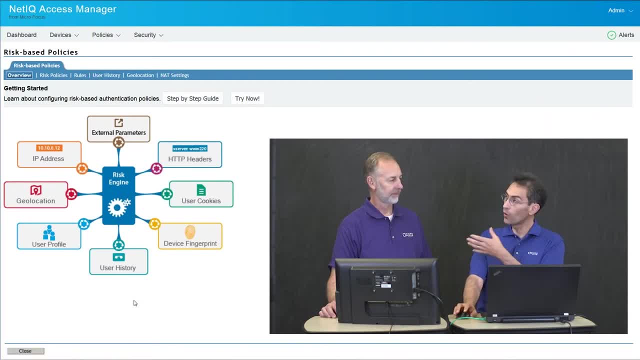 I'm going to let that pass. But user history allows us to look at your pattern of behavior, to add that in as an input to one of these rules, to see: okay, he hasn't done this in 30 days or 60 days, let's go. 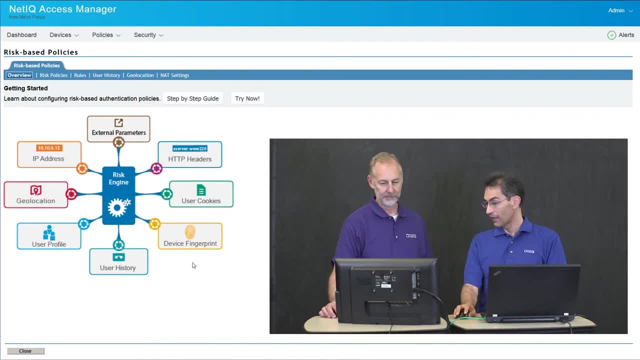 ahead and increase that risk level that we talked about. Device fingerprint is an interesting one, So I can fingerprint the device that you're using. each device that you use to access these resources, I calculate that fingerprint during the authentication and if it's a device I've never seen before, 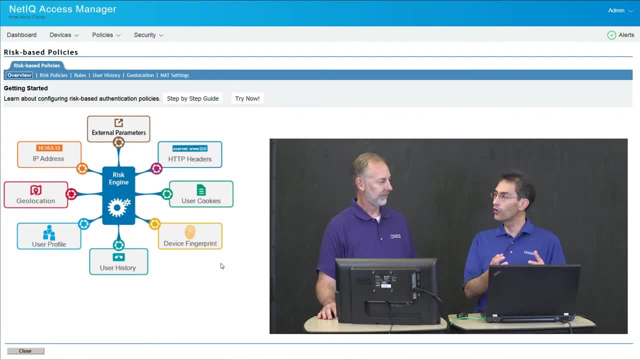 I'm going to again increase the risk, Increase my risk score, require you to enroll that device so that I can, or access manager can, identify this particular device associated with you, so that the next time I say, okay, it's Kent using the same device, okay, we'll let him through. 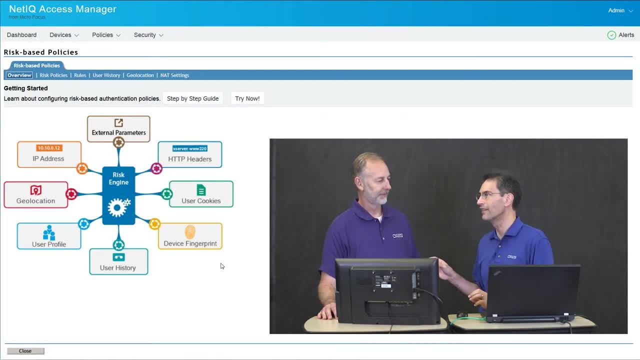 And the next time? oh, it's Kent using a different device. are we sure this is Kent, Right? So this is a way for us to auto to fingerprint the device, auto enroll you in that fingerprinting process. So, as opposed to making sure there's no risk, 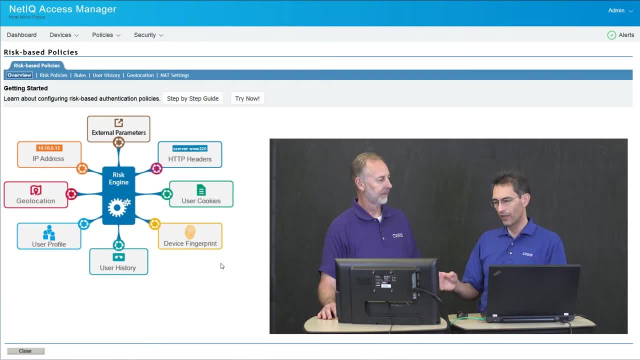 Making sure there's some nasty, stringent policy that you have to somehow grant access to that specific device and tie it to you specifically in another way. This is a lot easier way to do it. User cookies probably. there's a lot of use for it, but it's not as much as it used to. 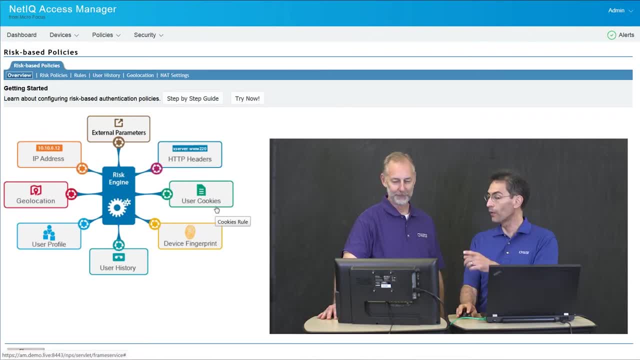 be. This is the old way of doing access and that sort of thing. but what's kind of cool about this is that access manager can build its own cookies, again based on the level of access, put it down in the workstation. we can use that too. 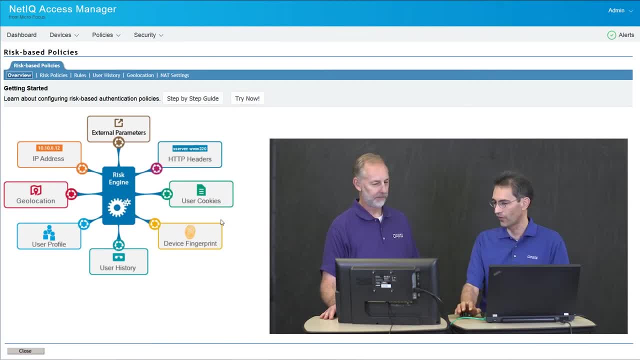 Because that tends to be ubiquitous- always works on every type of device scenario. Also, these types of cookies we can use. you can mint your own cookies in your own applications that we can look for as well. So you can build those rules too. 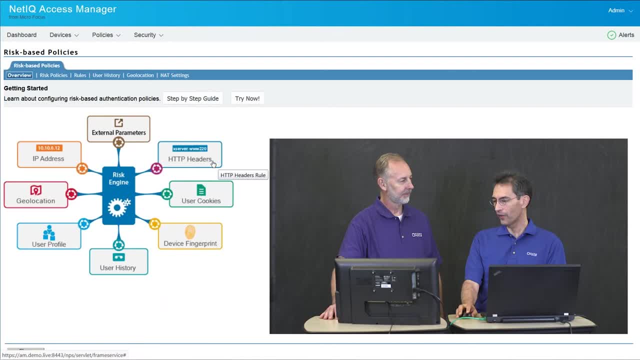 Yeah, HTTP headers is an interesting one as well. This one can be same thing. Your applications can put headers into the application that we can go look for, see if they're in there, what the values of those headers are, and use that as a risk posture. 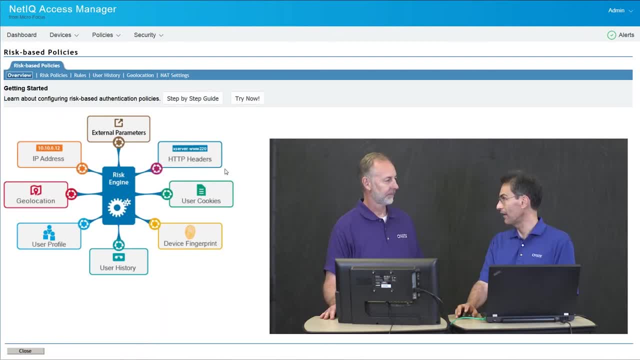 analysis tool as well. That can also be done at your network layer. So we talked about how the IP address can represent if I'm inside or outside the corporate network. Well, if your network infrastructure can inject a header, which this is commonplace, then 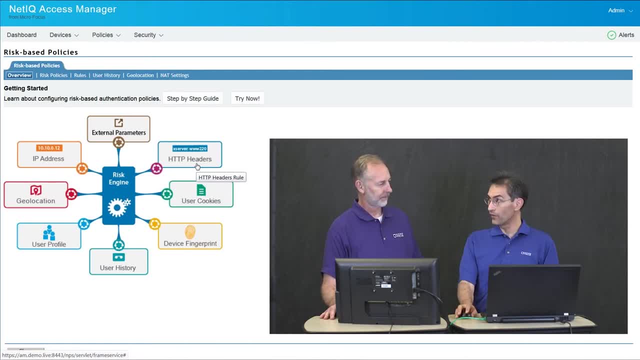 we can interrogate that header So we'll know that your actual physical network hardware went in, took a look at what you're doing and injected a header that we can look for as well. So it gives you another level of surety that that is who the user is. 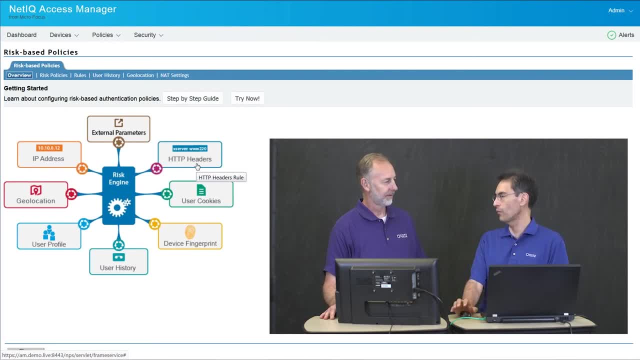 Who the user says they are and that's using it from a place that we trust. Right, Got this one on top External parameters. Yeah, It's the last one, even though it's up at the top, right? Yeah, The reason that I covered it last, even though it's up at the top, is: this is your golden. 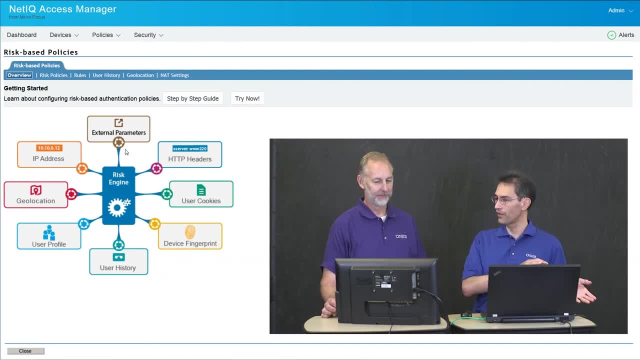 ticket to anything you want. This is the way you can reach out into other systems. We've had some customers reach out into the network hardware at a very granular layer and ask it questions that I can then use as an evaluation. So I can pull in any type of risk from other systems and pull that into this risk calculation.